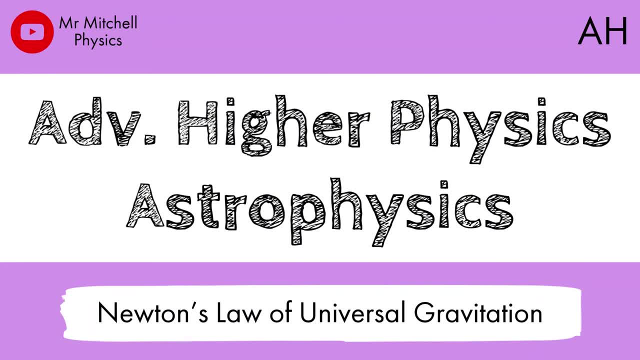 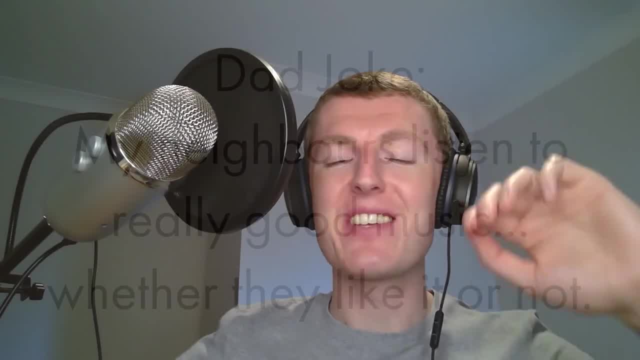 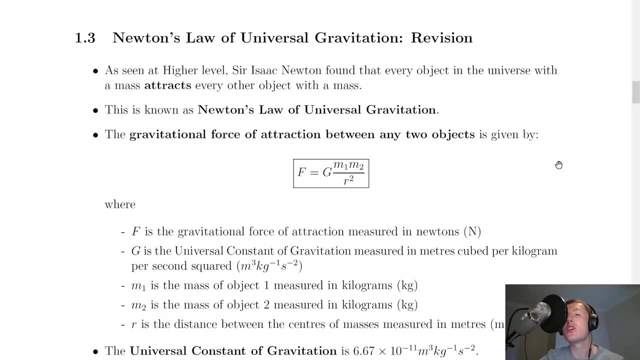 Hey guys, how's it going? In this video, we're going to look at Newton's Law of Universal Gravitation, So let's get started Now. you'll see that this is revision, because you should have done this in the higher physics course, and it says that, as seen at higher level, Sir Isaac Newton found that every object. 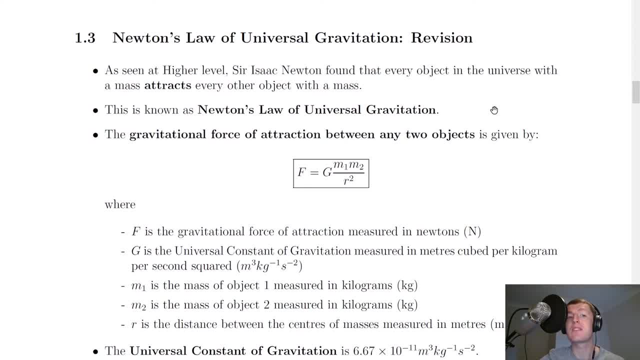 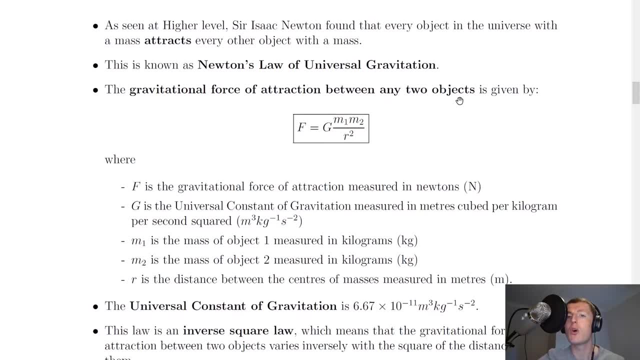 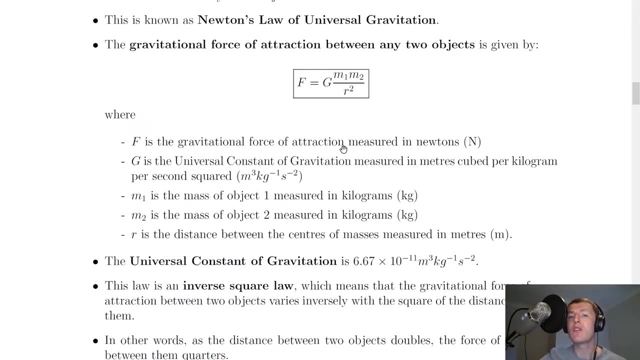 in the universe with a mass attracts every other object with a mass. This is known as Newton's Law of Universal Gravitation, and we represent the gravitational force of attraction between any two objects. with this equation here, F equals g times m1, m2 over r squared, where f is the gravitational force of attraction. 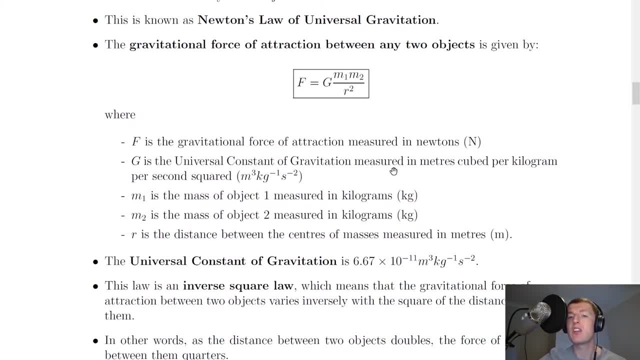 measured in Newtons. g is the universal constant of gravitation measured in metres cubed per kilogram per second squared, and that is on the datasheet in your exam. m1 is the mass of object 1 measured in kilograms. m2 is the mass of object 2 measured in kilograms, and. 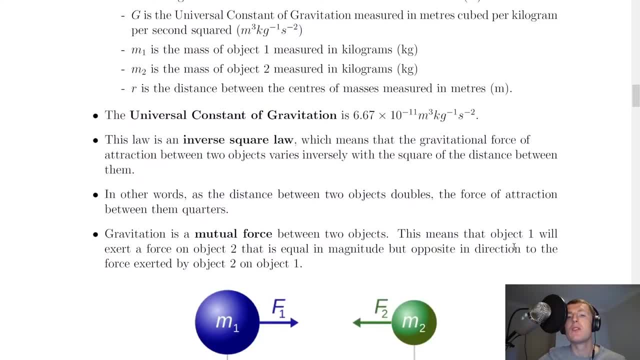 r is the distance between the centres of mass. So the universal constant of gravitation takes a value of 6.67 times 10 to the minus 11 metres cubed per kilogram per second squared. and, as I said, you don't need to remember. 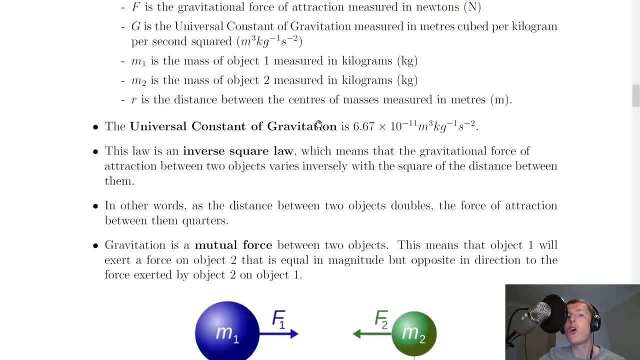 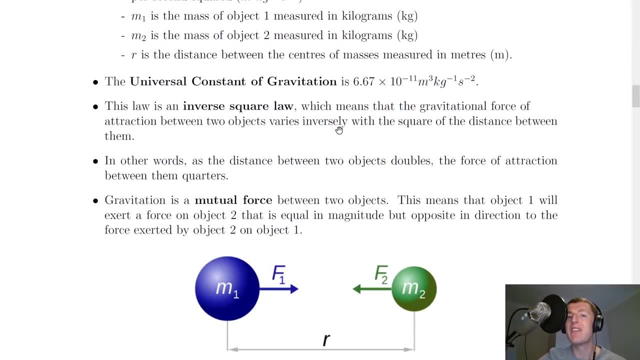 that number that is on the datasheet. This law is an inverse square law, shown by the 1 over r squared value there, which means that the gravitational force of attraction between two objects varies inversely with the square of the distance between them, or in other words as the distance between two. 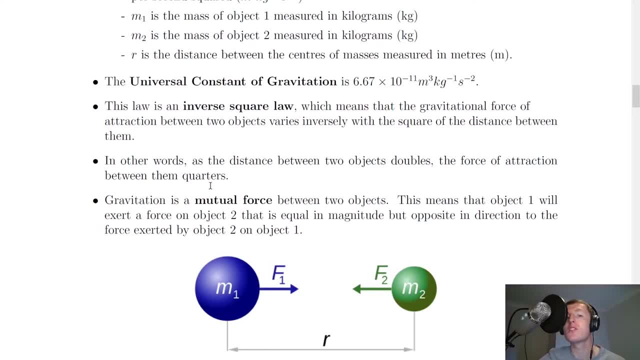 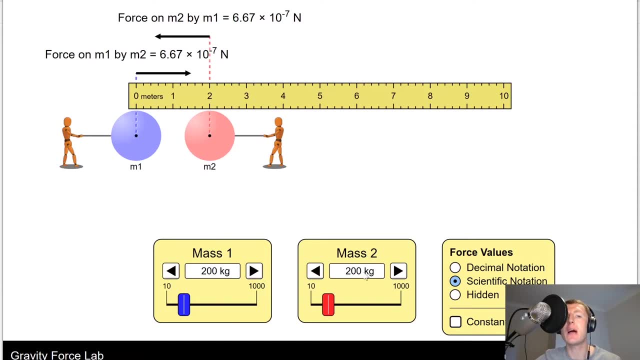 objects doubles, the force of attraction between them quarters. I'll show you a quick animation of this to help you visualise it. So here we've got two masses, m1 and m2, each of mass 200 kilograms, and you'll see. 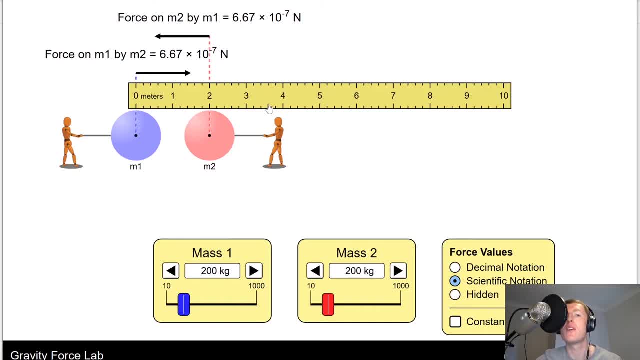 that each mass exerts a force on each other due to Newton's law of universal gravitation. So the force on mass m1 by mass m2 is 6.67 times 10 to the minus 7 Newtons, and we have the same value of the force for the force on mass m2 by mass m1.. 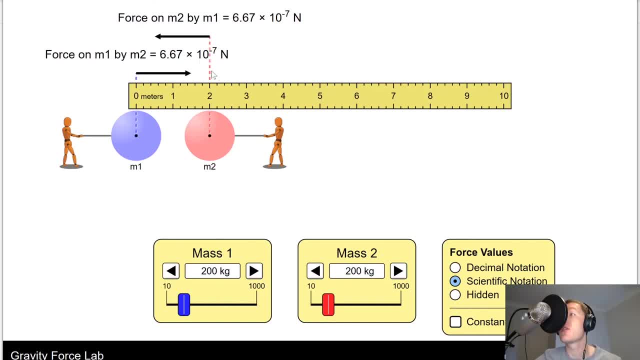 So this is like our Newton pair of forces here in Newton's third law, where we've got equal but opposite forces. You'll notice that the distance between the centres of the 2 masses right now is 2 metres. So when you divide by the distance given, by the distance between them, the distance between the 2 masses 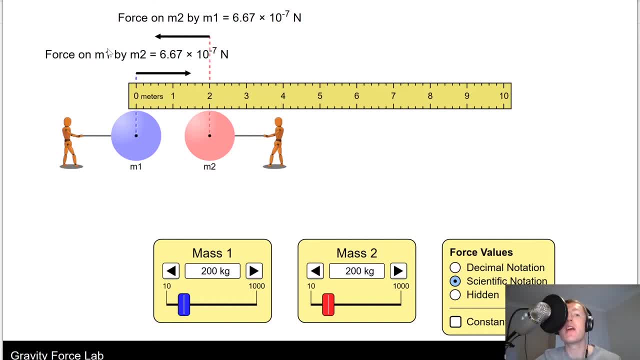 but if I was to double that distance then we should see that the force value quarters because of the inverse square law. So if we double the distance from 2 to 4m there, you'll notice that we are now at a quarter of the value of force that we just had, and you can. 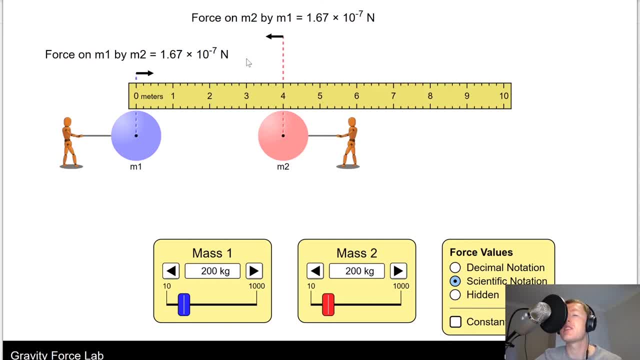 check that as the case. So we've now got force values of 1.67 times 10 to the minus 7N, And the same should happen again if we were to double our distance from 4 to 8m this time. 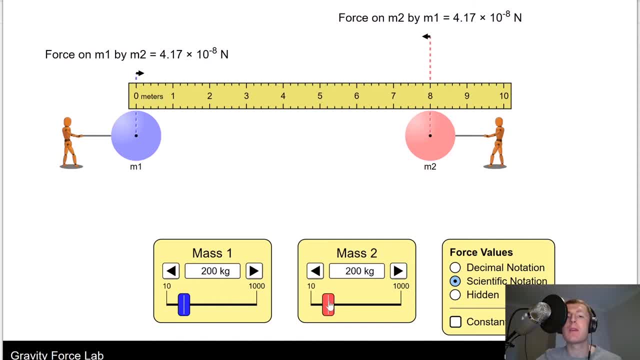 we should have our value quartering again from what it was just at. It should also be pointed out that the larger the mass, the larger the forces. so if I was to increase the masses there, you'll notice that our force value is increased And that's. 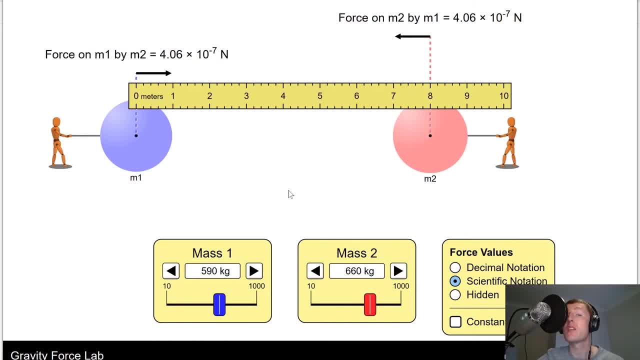 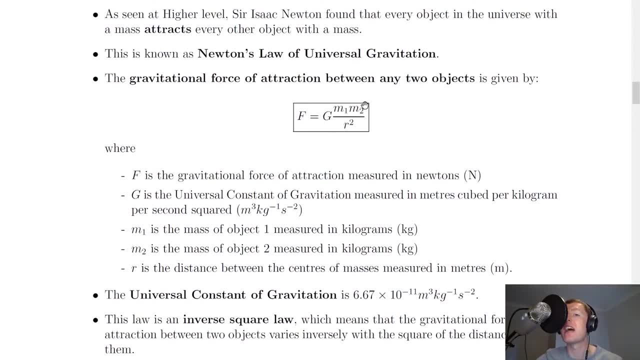 because the gravitational force of attraction is directly proportional to the mass of each object. Going back to the notes now, you'll see that in the equation- so we've got f is directly proportional to m1 and m2, because that's on the numerator of the equation and we've got. 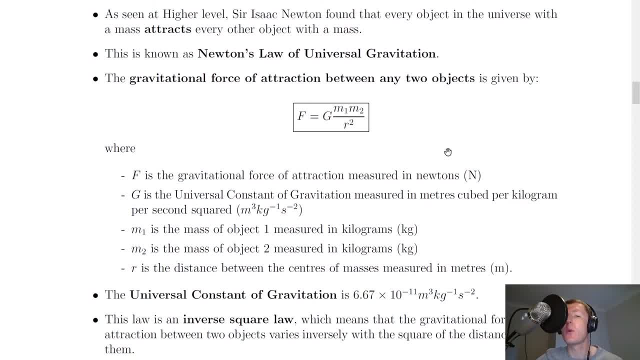 f is proportional to 1 over r squared, which is our inverse square law. Lastly, for this part, it says that gravitation is a mutual force between two objects. This means that the force of attraction is directly proportional to the force of attraction. This 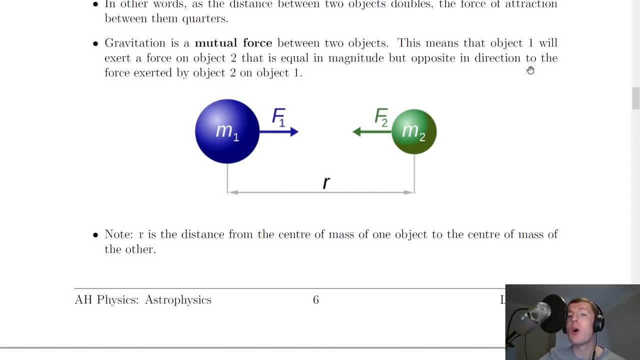 means that object 1 will exert a force on object 2 that is equal in magnitude but opposite in direction to the force exerted by object 2 and object 1.. So we've just seen that. so you have your force f1 acting onto mass m2 and your force. 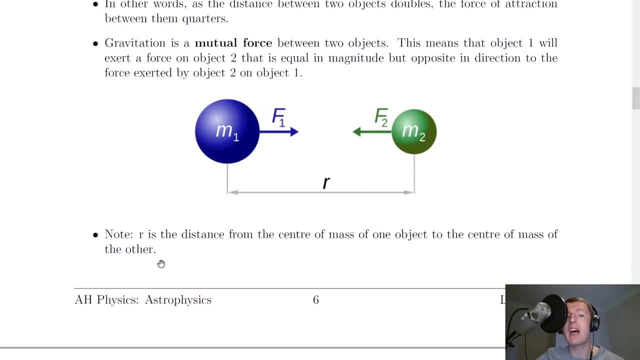 f2 acting onto mass m1.. And notice that r is the distance from the centre of mass of one object to the centre of mass of the other. so it's important that you're dealing with the centre of masses when you're doing questions. 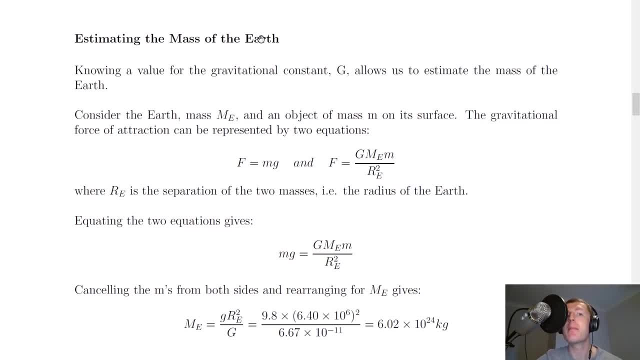 Newton's law of universal gravitation can be used in estimating the mass of the earth. So it says here that knowing a value for the gravitational constant g allows us to estimate the mass of the earth. Consider the earth of mass m, e and an object of mass m on its 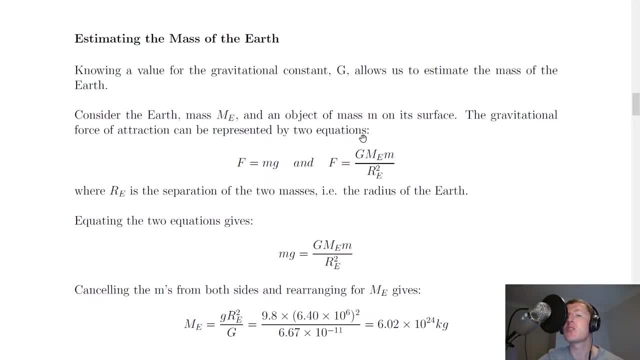 surface, The gravitational force of attraction can be represented by two equations. So we've got f equals mg, which is just another form for f equals m, a or w equals mg, where g is our gravitational field, strength or acceleration due to gravity, And f equals gm, e times m. 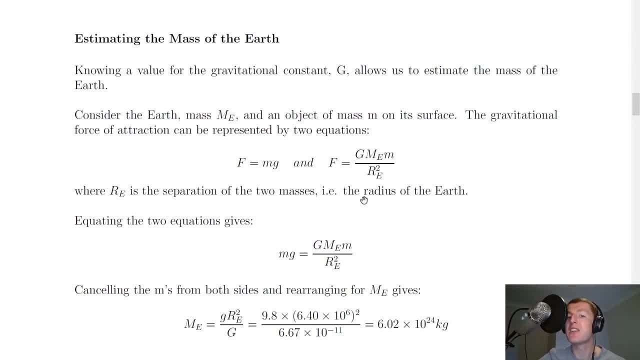 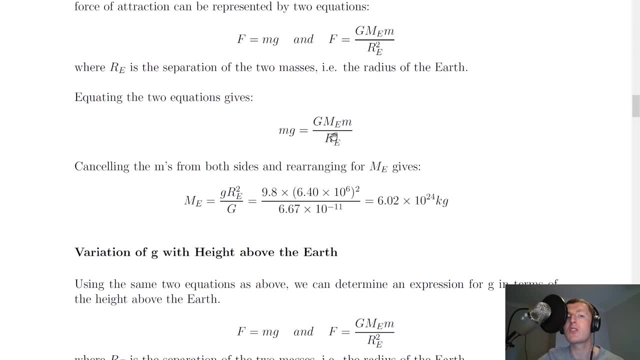 over r e squared, where r e is the separation of the two masses i, v and x. This is a formula, ie the radius of the Earth, And if we equate the two equations then we get: Mg is equal to G, Me times M over Re squared and you'll notice we've now got a small m on each side. 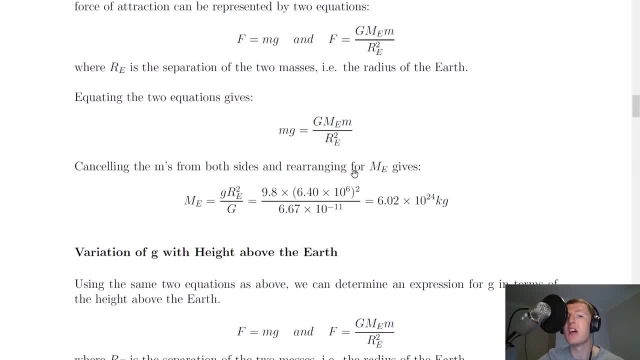 so we can cancel those out. and so cancelling the m's from both sides and rearranging for the mass Me gives Me is equal to G times Re squared over big G. and if you then substitute in the values for the gravitational field strength on the Earth, the radius of the Earth, 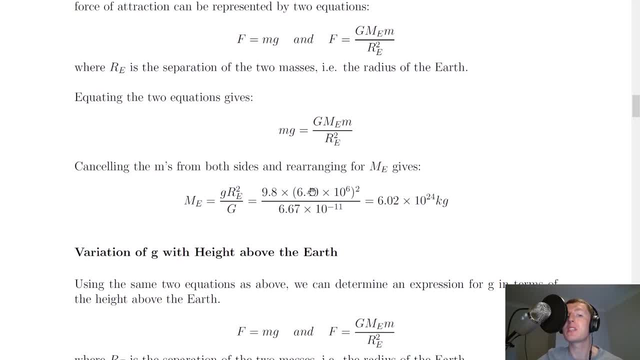 and our universal constant of gravitation, we get 9.8 times 6.40 times 10 to the 6. all squared, divided by 6.67 times 10 to the minus 11, is equal to 6.02 times 10 to the 24 kilograms. 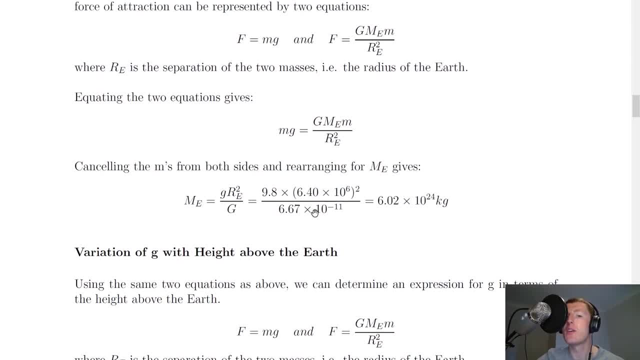 So, just to point out, you get this value of the radius of the Earth and the universal constant of gravitation on the datasheet in the exam, and you would also get this value for the mass of the Earth as well, but we've shown that we can estimate it using Newton's. 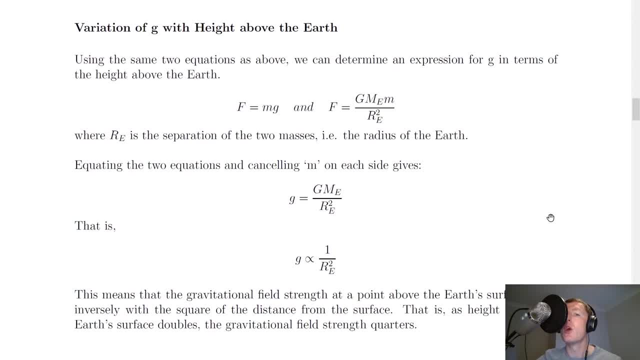 law of universal gravitation. Lastly, another thing we can do with Newton's law of universal gravitation is to calculate the mass of the Earth. So if we calculate the mass of the Earth, we can calculate the mass of the Earth and we can calculate. 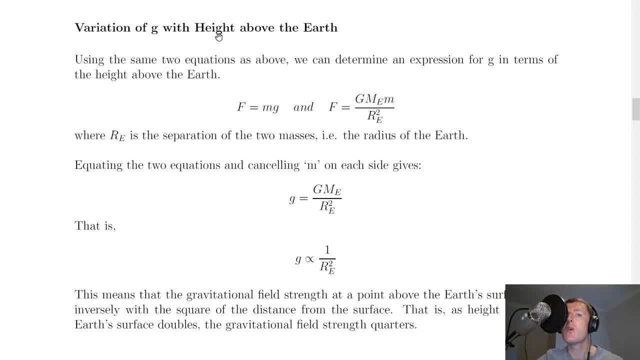 the mass of the Earth. So what we can do with universal gravitation is to look at the variation of gravitational field strength, G, with height above the Earth. So it says here that using the same two equations as above, we can determine an expression for G in terms of the height above the Earth. 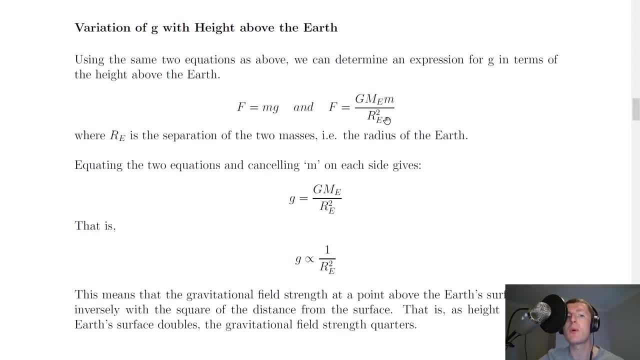 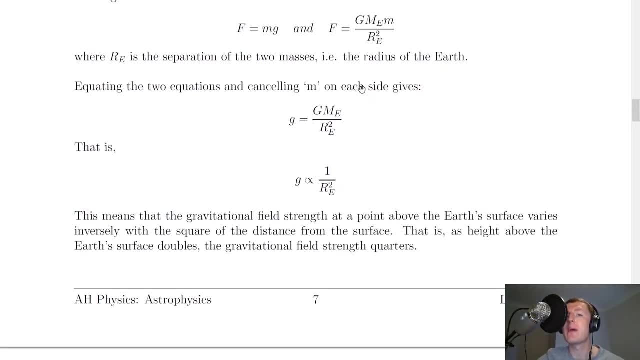 So F equals mg and F equals G. Me times m over Re squared, just like before, where Re is the separation of the two masses, ie the radius of the Earth. So equating the two equations and cancelling the m on each side gives small g equals big G times Me over Re squared and. 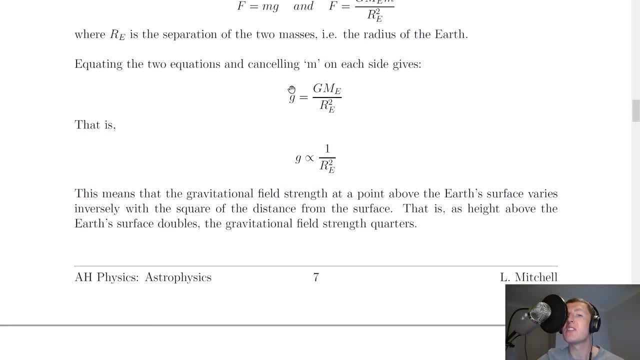 notice, this time we've not rearranged. All we're interested in here is the gravitational field strength, g and the radius of the Earth squared. So if we ignore the constant g and Me for now, we can write down this inversely proportional relationship here, which says that gravitational field strength is directly. 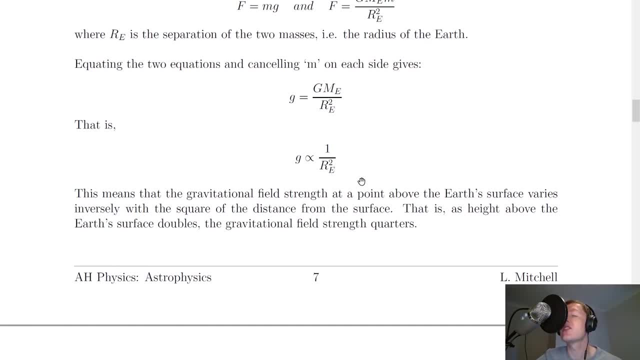 proportional to 1 over radius squared, And so this is our inverse square law. So this means that the gravitational field strength at a point above the Earth's surface varies inversely with the square of the distance from the surface. This means that the gravitational field strength with the square of the distance from the surface. 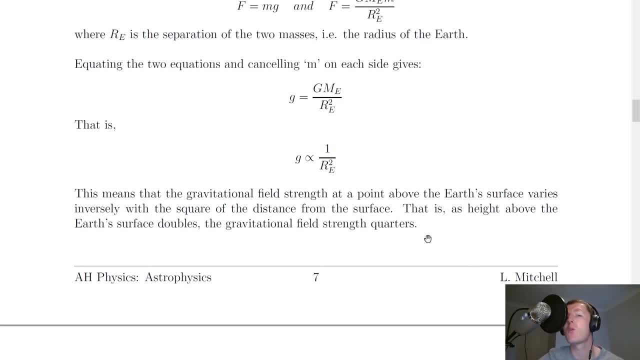 above the Earth's surface doubles the gravitational field strength quarters. Or in simpler terms, as the height above the Earth's surface increases, the gravitational field strength decreases, And we can show this using an animation. So if you ignore all of this text on the left,